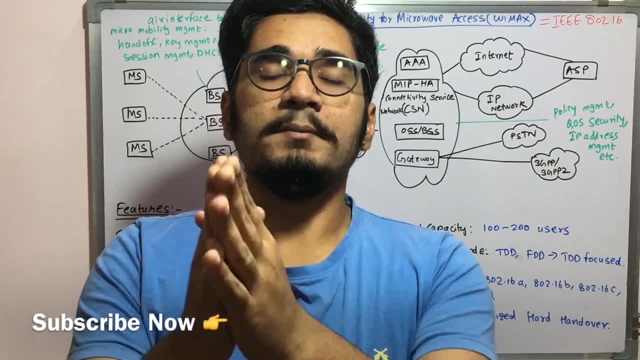 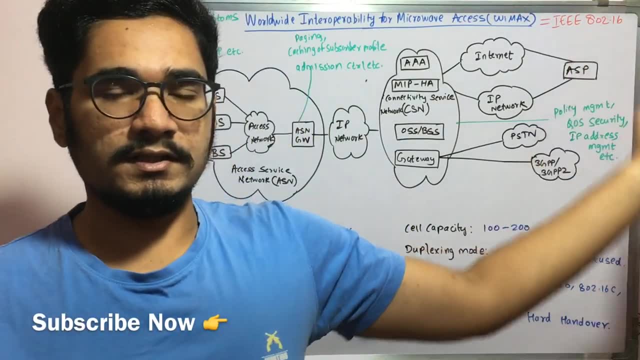 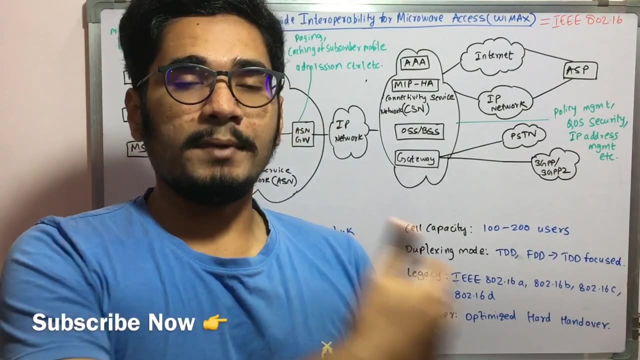 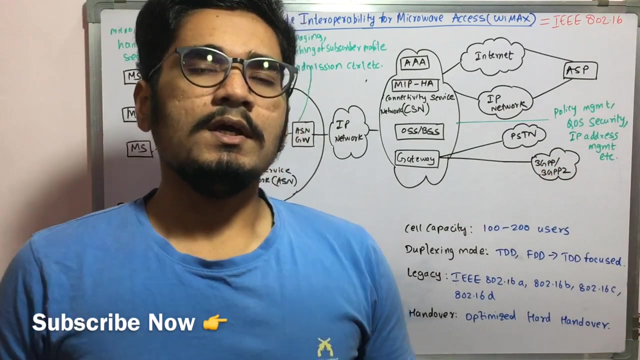 Welcome back to my channel. So today, in this video, let's see what is WiMAX. that is, worldwide interoperability for microwave access, which is also called as IEEE 802.16.. So many people have the confusion that whether IEEE 802.16 is actually a different technology or whether WiMAX is called as a different standard. but no, it's the same. You have IEEE 802.11 for WLAN as well, So just a name given by the IEEE standard, just for convenience, just to separate it as a 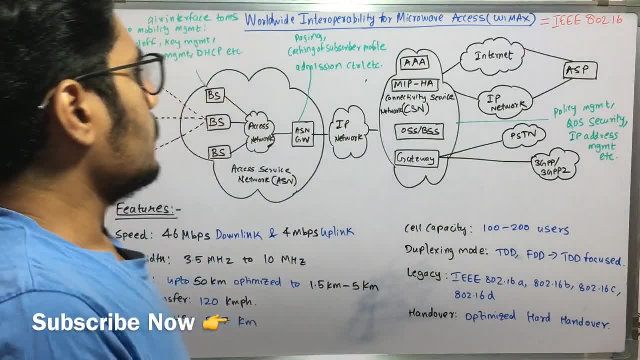 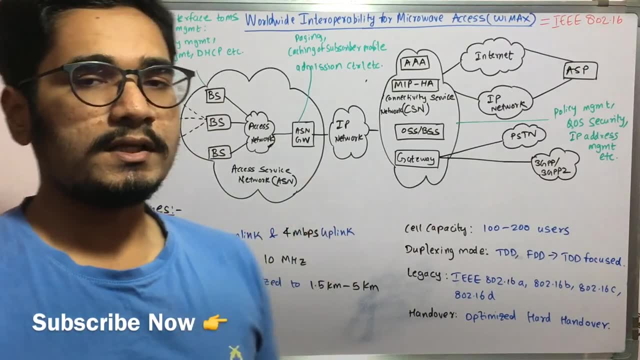 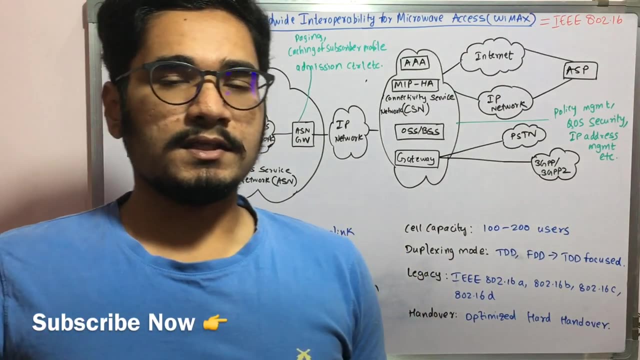 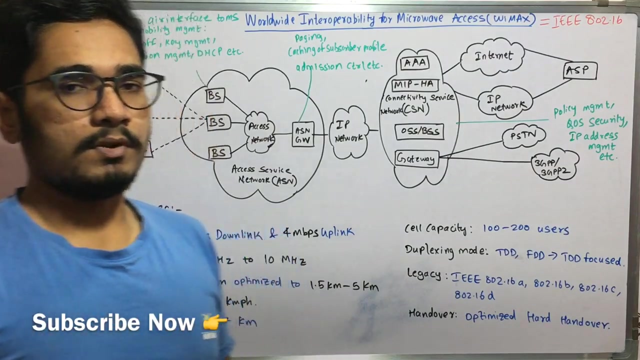 different technology from all the different technologies. So in this video let's see the IP architecture, or IP based network architecture of WiMAX, how it looks like and what are the various components which are included in it, and some of the basic features of WiMAX, what it provides and some of its capabilities. So let's begin. So we have this entire big architecture. So this is an architecture based upon the IP, So IP is mainly functional in this, throughout the entire architecture. 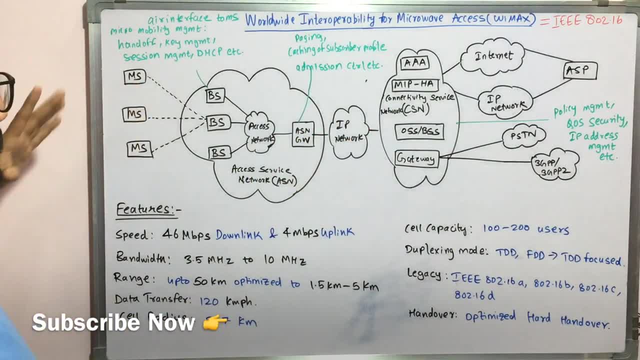 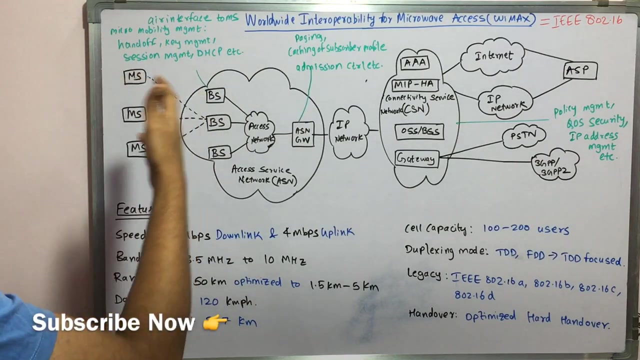 So to begin with we have this MS, that is, mobile stations. So mobile stations are connected to these two layers. So basically the second layer in this is the access service network and then you have the connectivity service network, CSN, So this mobile stations are connected to this base stations via this air interface. So base stations mainly provide an air interface to mobile stations and also it participates in some kind of micro mobility management which provides handoff and 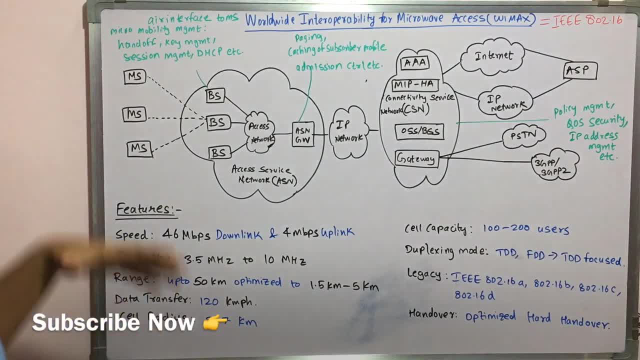 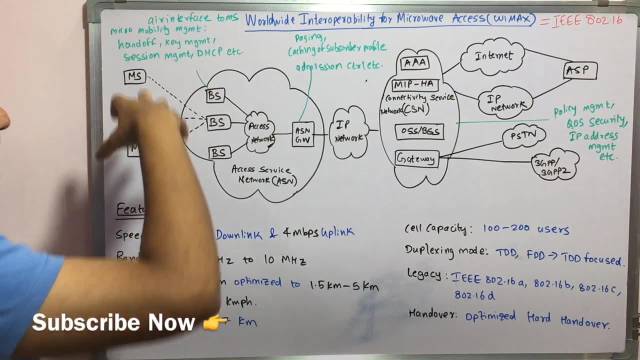 then key management is there, some translations are there. then session management, dynamic host configuration, protocol, resource management- many functionalities are provided by this base stations. then you have this access network. so access network just collects all the available base stations which are there, that particular ASNs, and then it forwards to this ASN GW. that is access. 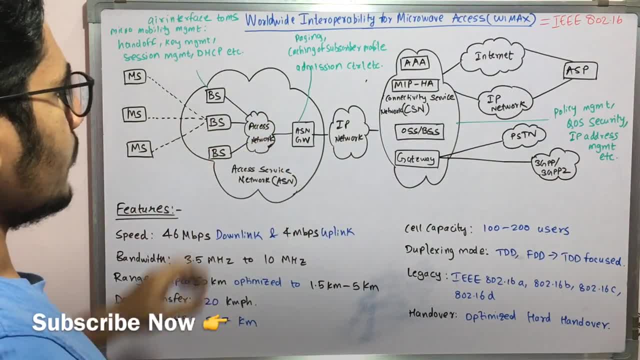 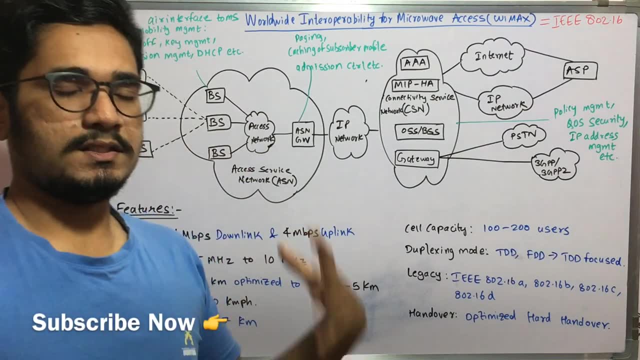 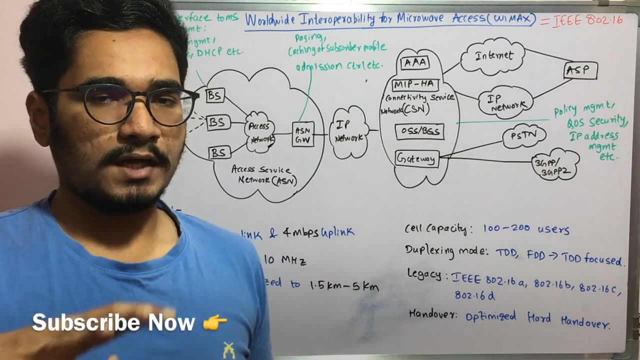 service network gateway. GW is for the gateway. the major functionality of this part of this model is the paging: paging of all the devices or all the systems which are there in the WiMAX and then caching of subscriber profile. so basically, there are n number of subscriber profiles or subscribers who might be registered to the WiMAX system. so whenever, if any new access or 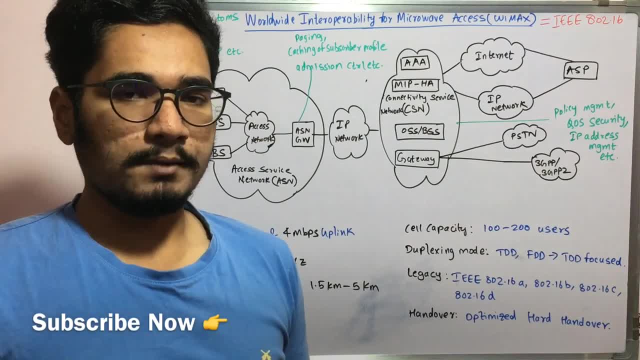 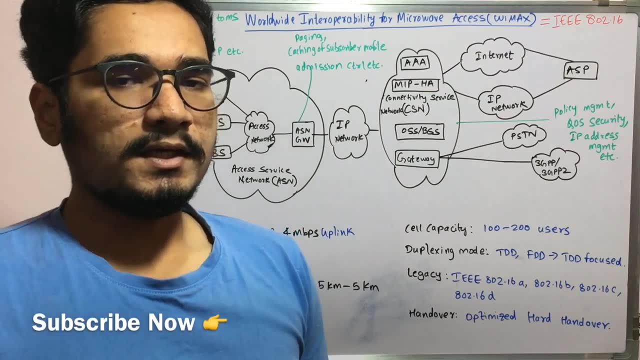 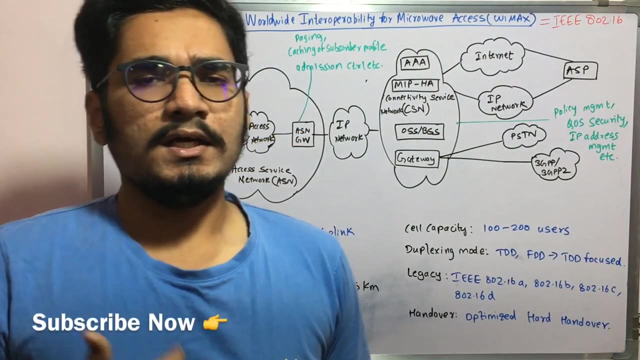 if any new request from already existing subscriber comes, then it will just update it from its cache, else it's a new customer, then it will be dynamically creating that particular subscriber profile. next you have the admission control. so admission control is nothing, but just the rule whether the 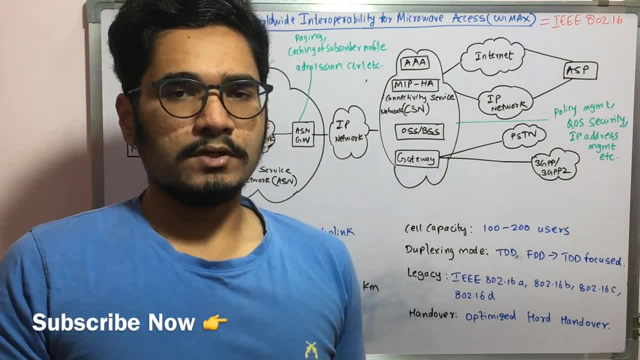 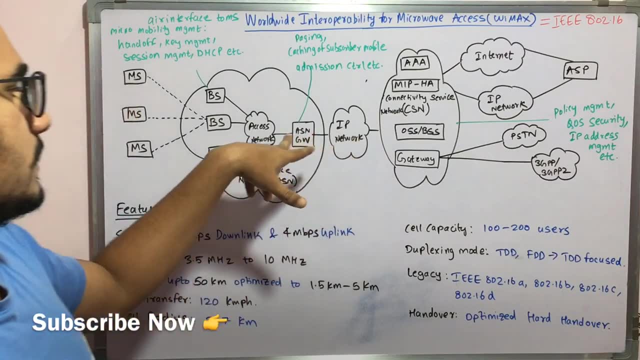 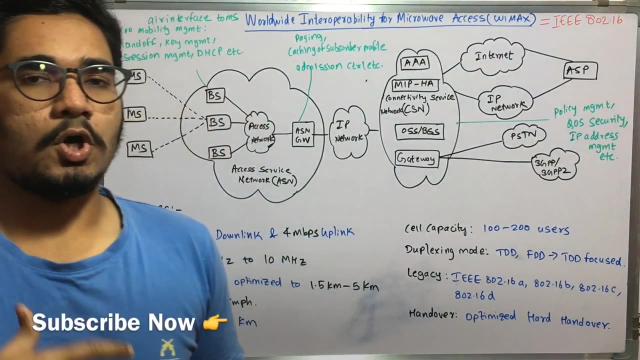 proper IP packets or whether the proper request should be sent or not, because it mainly concerns with all the legal issues and major security is just kept over this ASN GW. then further we move on. we have this IP network. so IP network is basically consisting of all the list of IP. 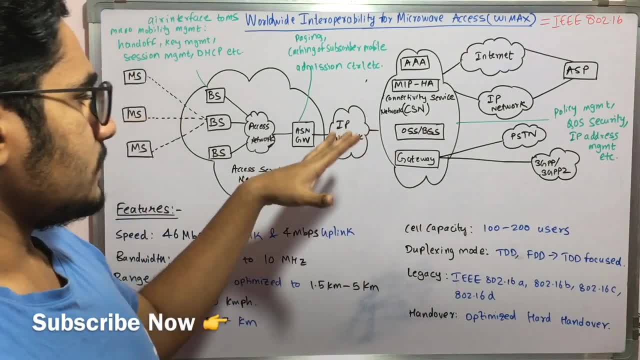 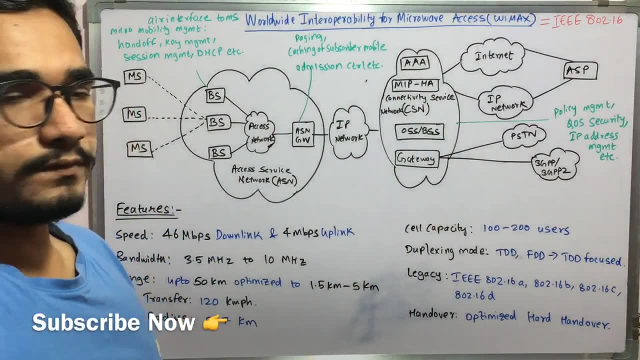 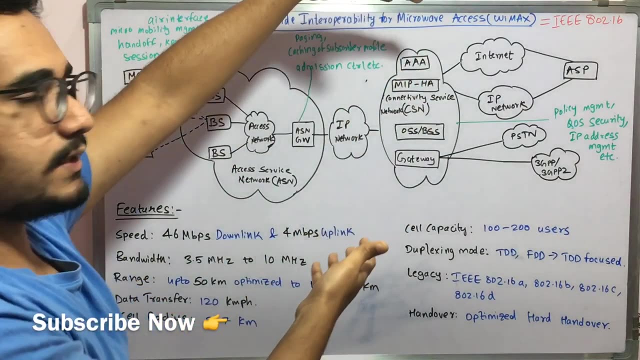 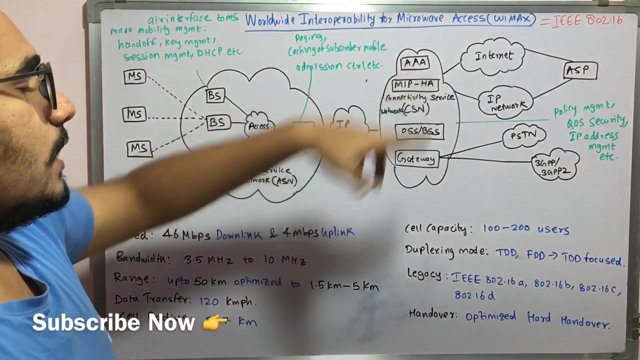 addresses which are there, all the whitelisted IPs which are there, which are listed as IP addresses, which are just triggered for forwarding of all the requests. then you have this connectivity service network which actually connects all these particular various technologies, in fact all you can see various technologies. so we have this AAA, that is, authentication, authorization, and 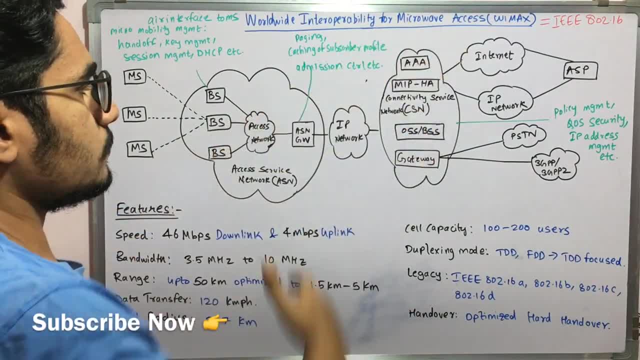 auditing of the resources which we have in the cloud resources. with this you can, just As Can, Use these. next is connected it with this PL spider. next is job port root data, obviously. second last is the miteinander, naturally. the third is a network which has connected the data with this network app. it can detects the status, sir, the network, and instead of thatev Или, bedeutet that the right check between this network, or you can see that if it directly through it, then you have the network that is connected, simply a user, which is actually an amazing, a dedicated, knowing futures, which is specifically��, were 2434 and this link. that example is: 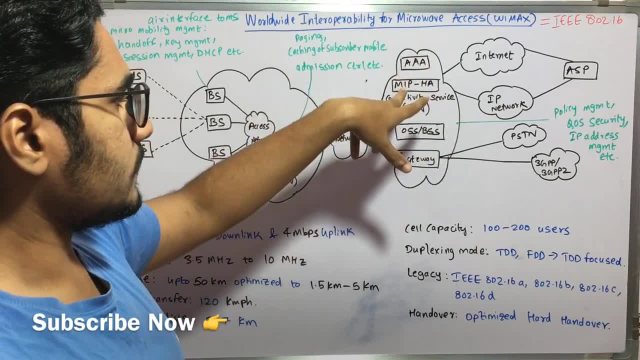 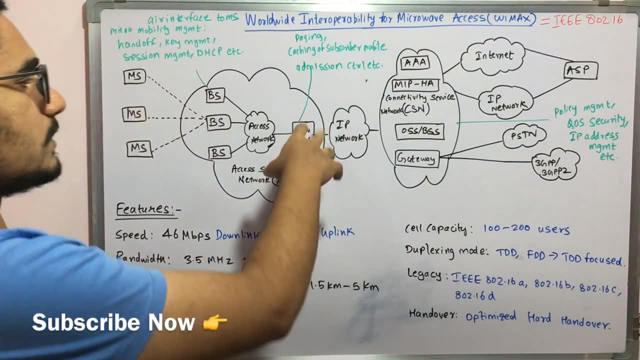 authorized dead server. so that means you actually can proceed. if you might simply mobile ip home agent, that agent is kept over here. that is only the home agent, where you need to just identify the original address of the current ip which comes on this ip network. so this contains: 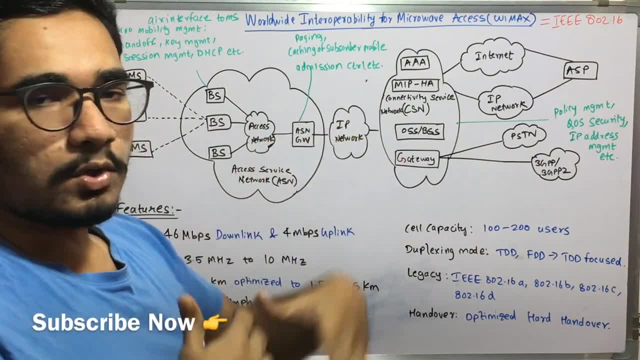 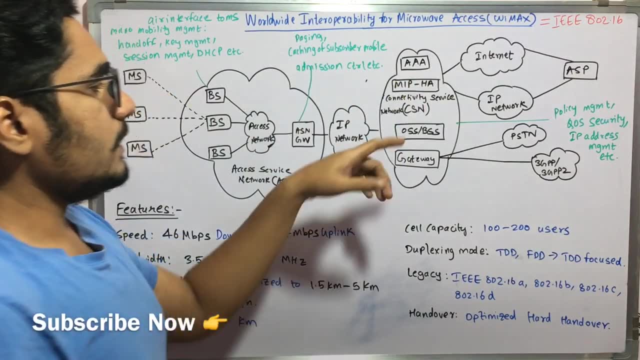 a pool of ip networks. so when, at a time, uh not all the ips would be coming, but only one particular ip would be coming here and just doing its activity, then you have the uh business support system, bss, and then you have the operation support system, which is used mainly for uh business activities. 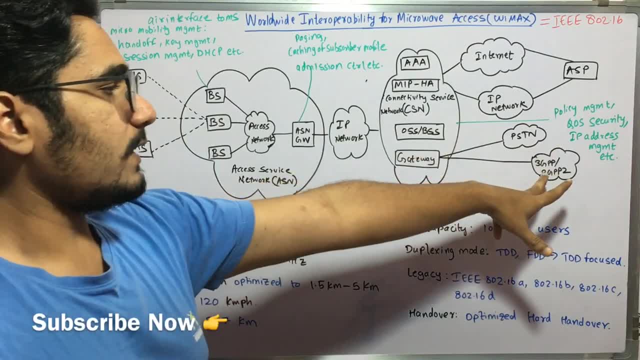 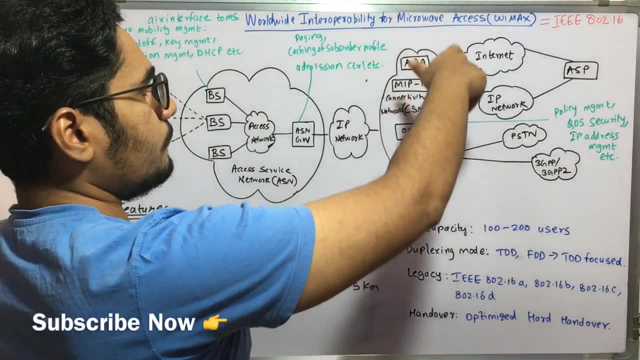 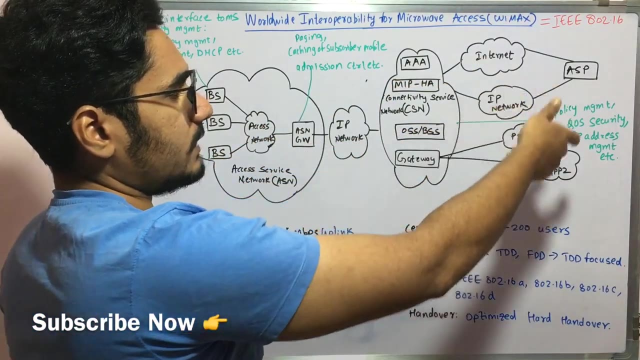 and then you have the gateway, which just connects to the pstn as well as 3gbp. that is, third generation partnership protocol and its supplanted version, 3gbp2, whereas if you move above you have this aa and mip connecting to the internet as well as the ip network. so there is a second layer of ip. 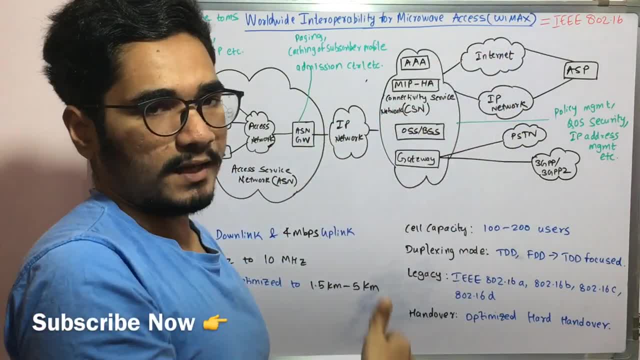 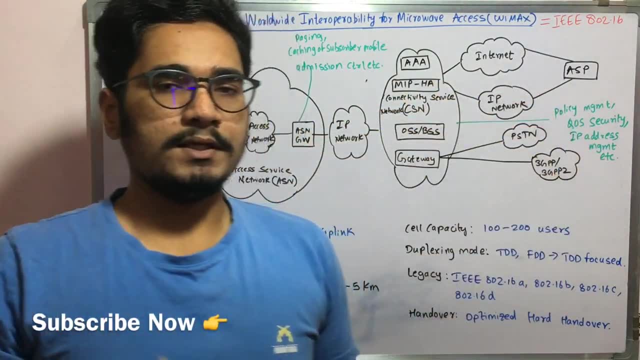 network over here which just rules or filters the proper ips from here, and then it's connected to the asp, that is application service provider. so there you get the front-end application to view all your applications- uh, regarding what all transactions you have done, or what all data. 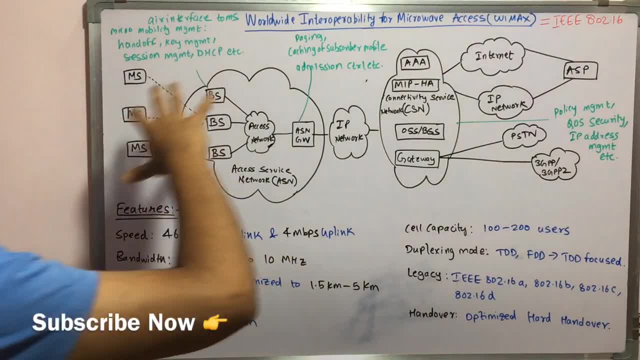 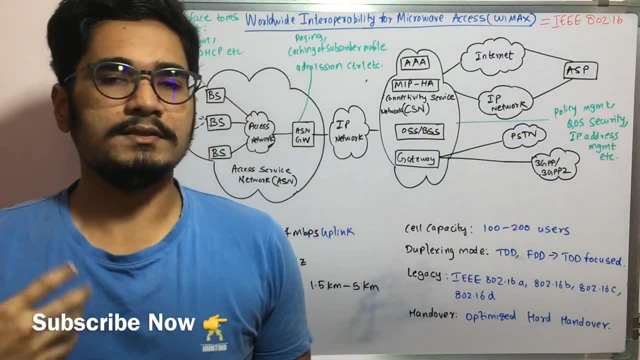 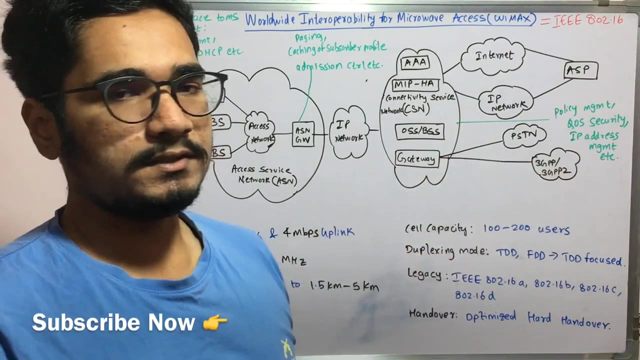 transfers you have done over the vimax system. so uh, this uh mainly connectivity service network. uh deals with the policy management, different policies of the users, whether he is able to read, write or access different resources over this vimax systems and the quality of service security is there, whether the proper handoff is done or whether the call is getting dropped or. 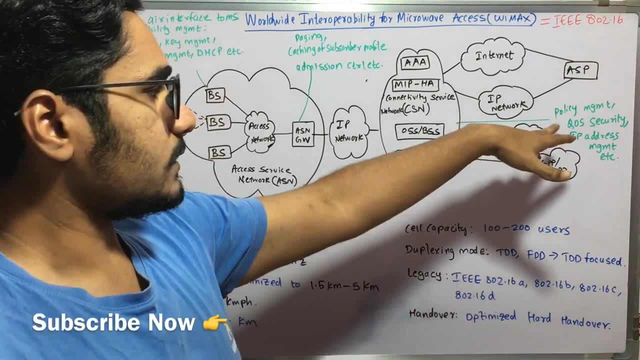 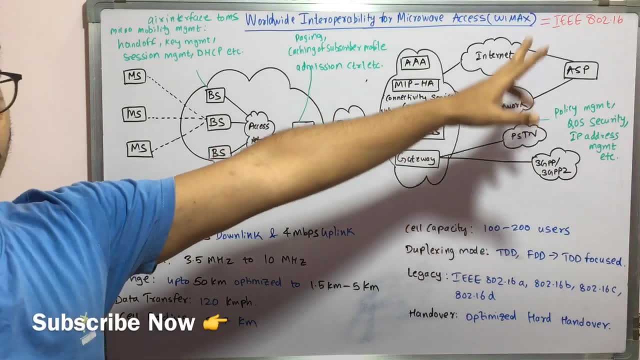 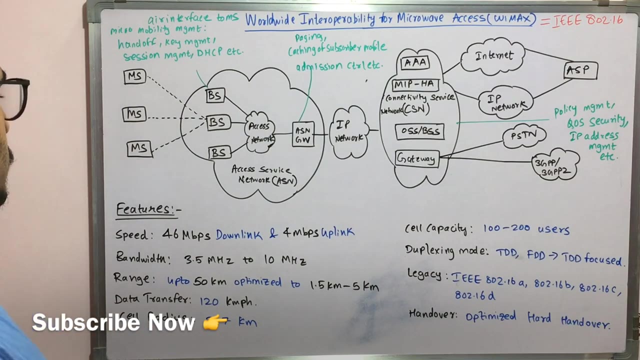 the different strength and weakness of that particular user is seen over here. then you have the ip address management. different ip addresses are managed over this network which is then forwarded onto this application service provider. so let's see some of the features which are there or which are possessed by the vimax system. so basically we 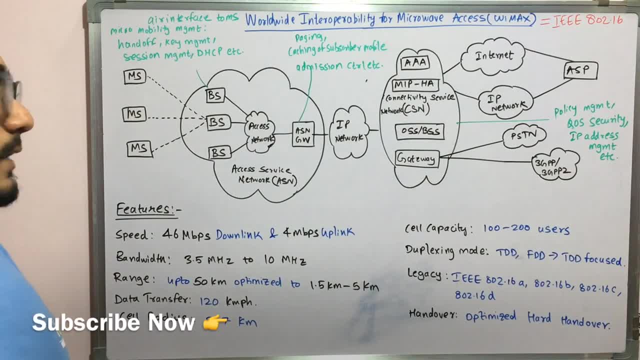 have taken nine different features. so very first is the speed. to talk about the speed, the downlink speed of imac system is about 46 mbps and the uplink speed is about 4 mbps. then you have the speed of the vimax system, which is 3.5 megahertz to 10 megahertz. uh, that's a normal range, uh, which? 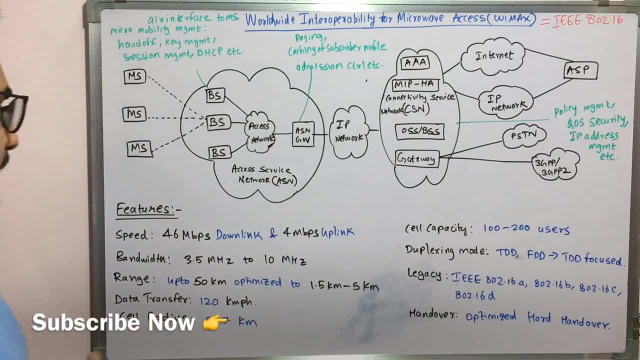 vimax provides. and then you have the range of the range. network connectivity is up to 50 kilometer, but it is optimized up to 1.5 to 5 kilometer by reducing the cell size, and so you have the data transfer has 120 kmph and then the cell radius, or the cell which you see in the co-channel interference. 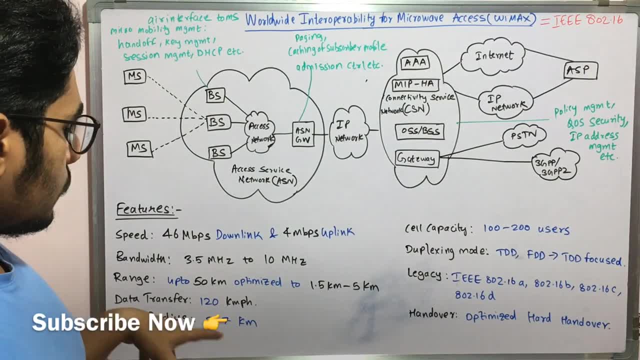 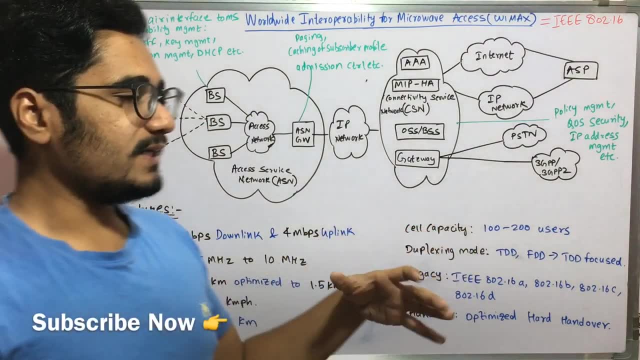 the d and the r parameters that cell radius are: r is about two to seven kilometers in this, and then you have the cell capacity means the entire cell in which vimax system operates. it can support up to 100 to 200 users per cell and the duplexing 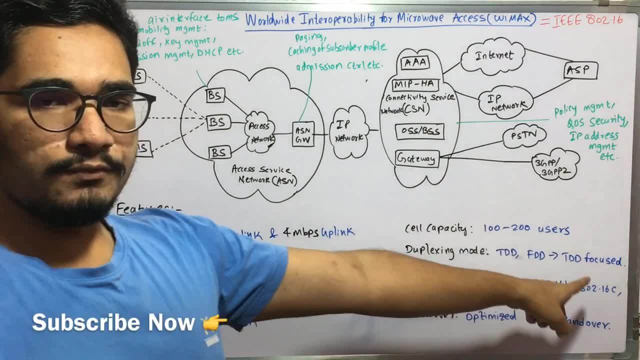 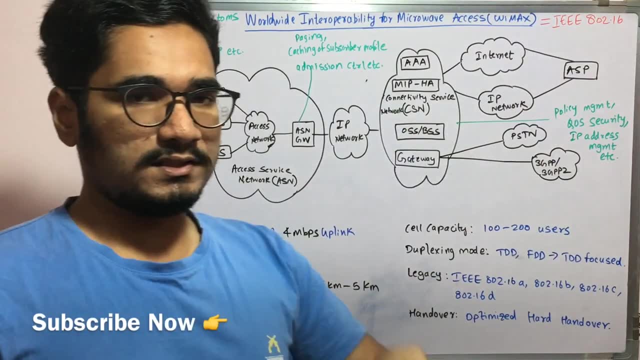 mode used in this is either tdd or upd, but it's mainly focused on tdd technology, that is, time division, duplexing. next up, the legacy protocol. so legacy is actually the standards which are there or which are seen in uh iwe 802.16, so it has 802.16.